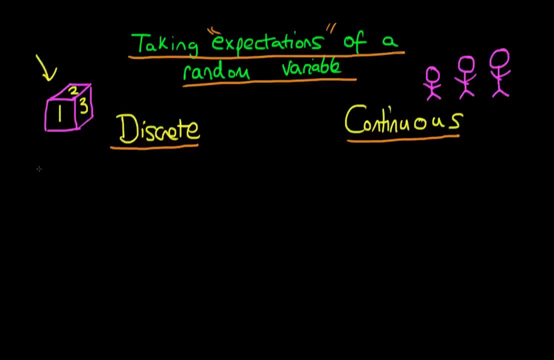 fair die. if you don't know, it is this sort of thing I've drawn up here in the top left, and it's a cube which on each of its side has written a different number, where the numbers go from one to six. So perhaps our random variable, x in this case, might represent the value which we obtain. 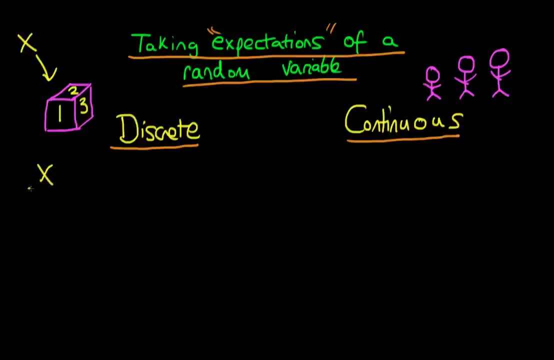 from throwing a fair die. So our sort of random variable can take on one of six values, starting at one, then go to two, three and then sort of continuing all the way up to six. So those are the sort of values which our random variable can actually take on and then associated with each of. 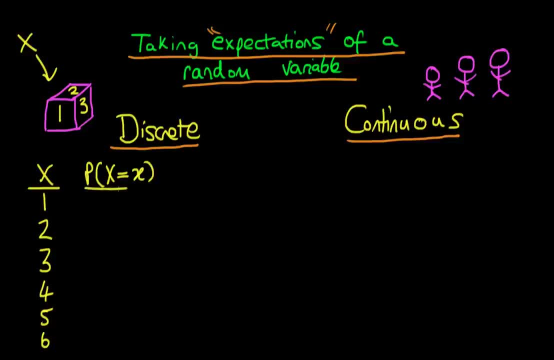 those particular values is a probability. We've written the probability that the random variable actually takes on that value. so here we've written the probability that big x, our random variable, equals little x, where little x represents the particular value in question. So the sort of first value here, the probability that 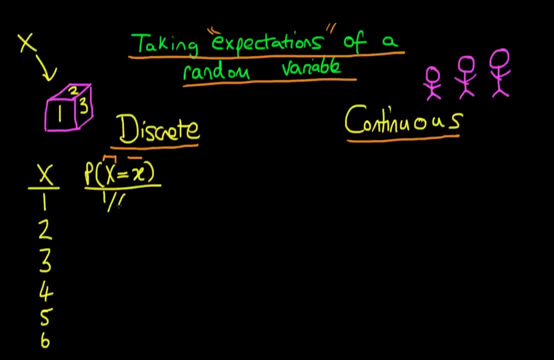 x equals one in the case of a fair die, this is just one over six. and the probability that x equals two is just one over six. again, probability that x is three is one over six, and we sort of continue likewise all the way up to six. 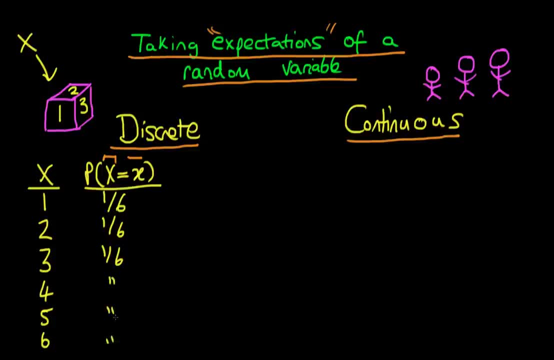 down to six. Okay, so that's sort of defined our problem. How do we then go about finding the expectation of our random variable, And what do we actually mean by taking the expectation? So the way in which we sort of write it is the expectation of a random variable, x, And in the 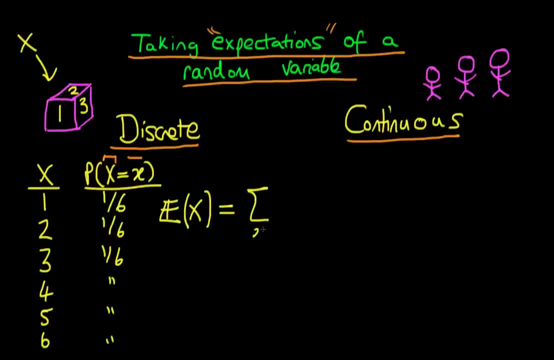 discrete case, this is equal to the sum over all particular values which our random variable can take on. So notice here that I've written little x to represent the sort of values one through six. And then the sum is the probability that big x equals little x. So the probability that a random 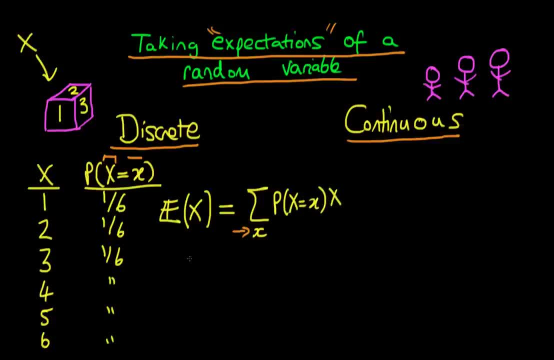 variable takes on that particular value times x, times that particular value. And so what does this actually mean? Well, the expectation is the sort of value which we would get, on average, if we were to roll our die a large number of times, or sort of, in practice, really, an infinitely number. 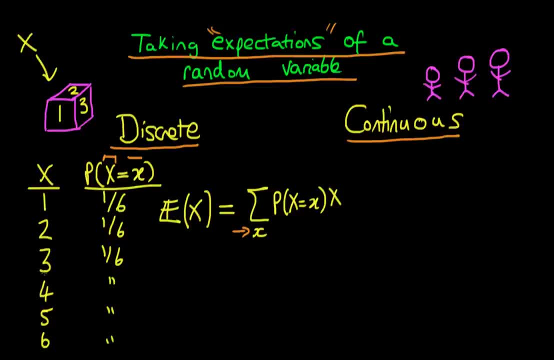 of times. So that's the sort of average number that we would expect to get on our die if we took a random variable x. And then the expectation is the sort of value which we would get on average if we took the average over all of those throws. But we can sort of use intuition. We don't need 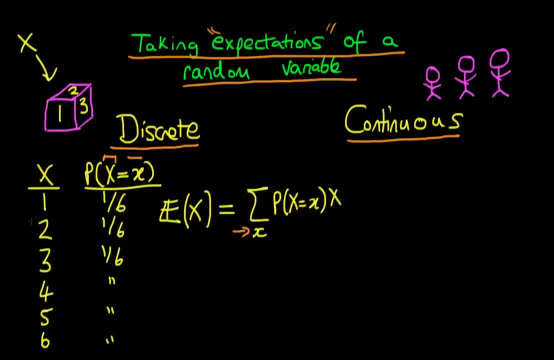 to necessarily use a formula to calculate this right, Because we sort of know that it's going to be halfway from the top and sort of halfway from the bottom. So it's going to be between three and four, And in the case of a fair die, rather, it's just going to be three and a half, And that's kind. 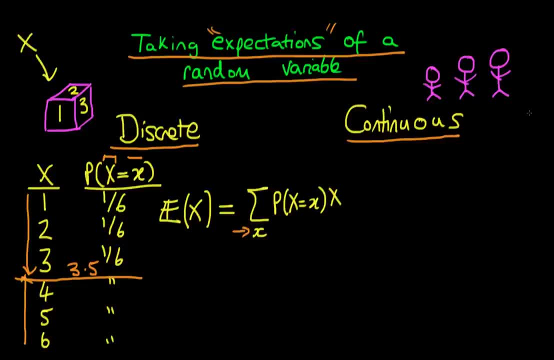 of quite easy to see just because of the way in which we've written this list here, But in sort of more complicated problems it might not be so easy to see what the actual expectation is going to be. Okay, so that's sort of using intuition. How do we actually go about finding? 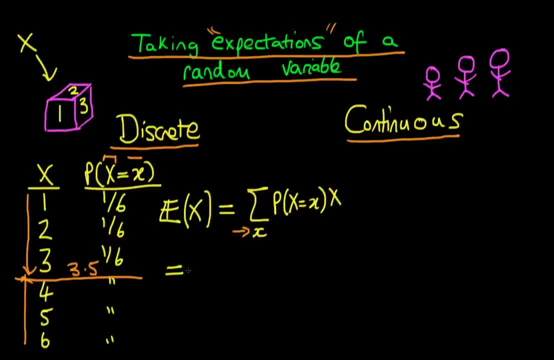 this value three and a half, using the sort of mathematical way. So if, just applying this formula, we have the first thing is going to be the probability that our random variable x is equal to one, And then we're going to have to multiply it by this x up here. So in this case, 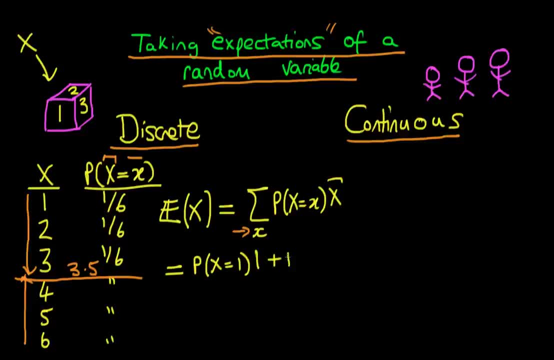 it's just going to be one, And then the second value is going to be the probability that our random variable takes on. the value x is equal to two, And then we're going to multiply that by two, because that's now the value which our x takes on, And we're going to sort of continue. 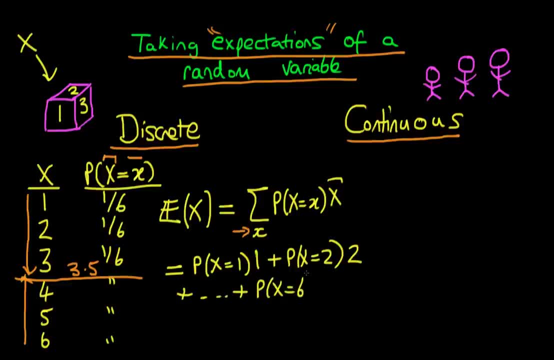 this all the way up to the probability that x equals six times six. And in this sort of fair die, because we sort of defined all these probabilities here, each of these probabilities is the same, So it's just one over six times one plus one over six times two, sort of plus one over. 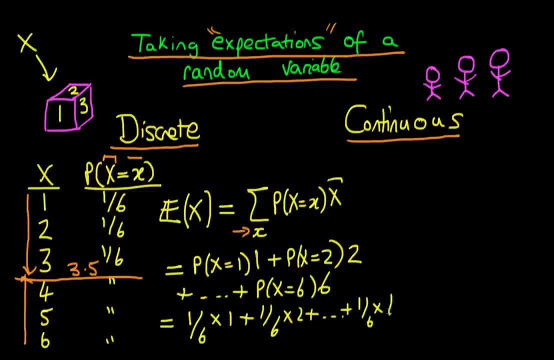 six times three, all the way up to one over six times six, which, if you do the maths, just adds up to 21 over six. Okay, so that's a sort of discrete case, But- and we've talked about what the actual formula is- But what's the intuition behind this particular formula? Why do 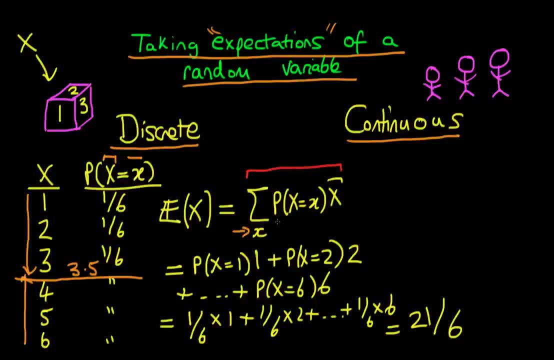 we actually use this sort of formula here. Well, you can sort of think about this as a weighted sum. I mean, if this probability wasn't here, then it would just be a sum over all x, So that would just be literally a sum over all x values. But these probabilities actually provide the 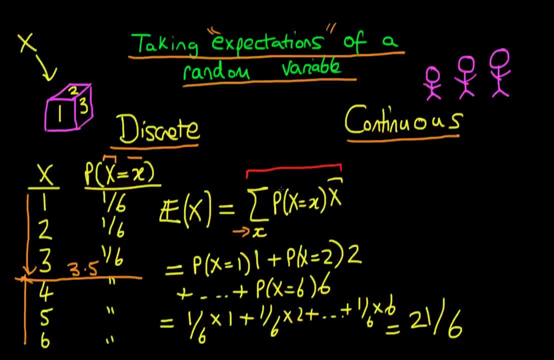 weighting in that sum And it just so happens that all the weights were the same in this particular example. So all the probabilities were the same in this example. So that's kind of the logic behind why we got three and a half, because it's sort of halfway down our list. But in general the probabilities won't be. 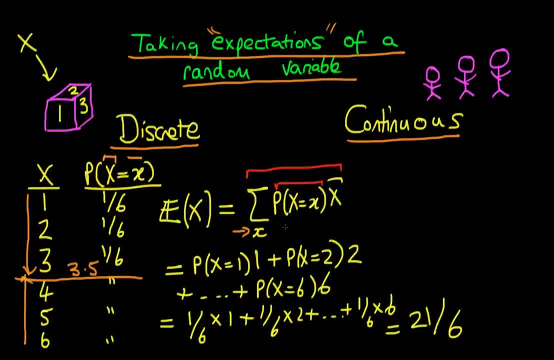 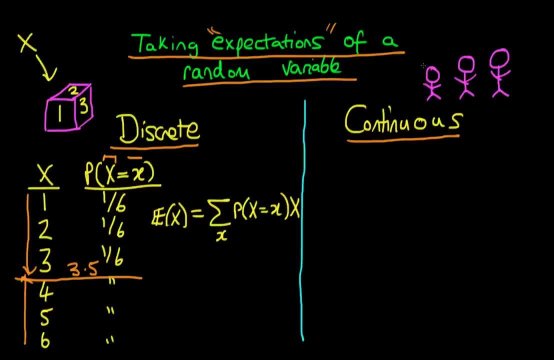 the same, And the sort of weights which the probability is applying are sort of intuitively, sort of providing more weight to those observations which are more likely to occur. So that's why you can use this formula to calculate the expected value of x. So I've rubbed out some of our working on the left hand side and rewritten the formula for the. 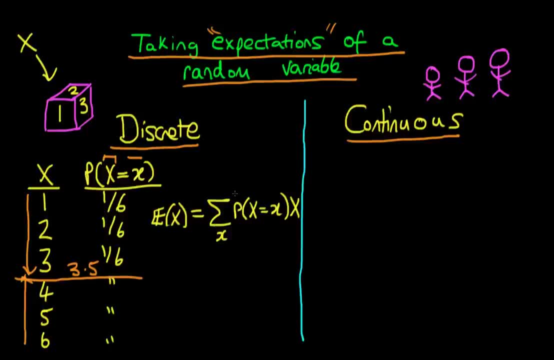 expectations, such that we have enough space to write out the expectations of a continuous random variable on the right hand side. So what is an example of a continuous random variable? Well, the example which I've tried to indicate here, with these sort of stick men at the top, is the example. 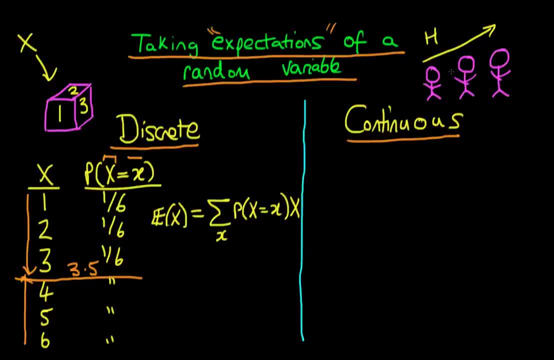 of taking the height of a randomly selected individual within a population. So we might think that the sort of frequency distribution which we might get in this case might sort of be normally distributed around some sort of height. So perhaps the sort of average height in a population is 150. 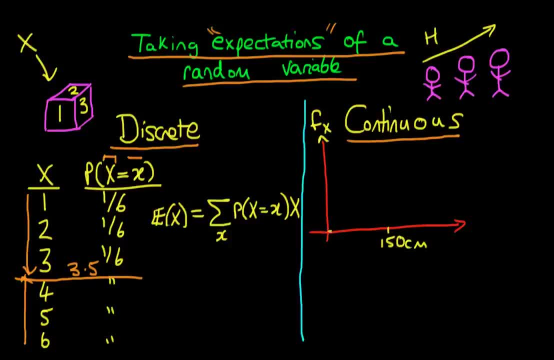 centimetres. So perhaps the PDF might look something like this, where we've sort of got our distribution centred around 150.. So how do we go about working out the expectations of the case where we've got a continuous variable or a continuous random variable? So we have a PDF representing the probability of obtaining 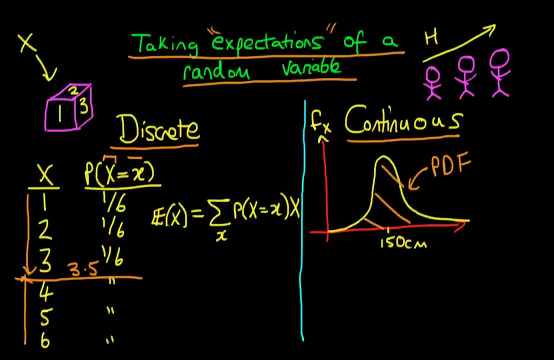 particular values across all continuous space. So how do we calculate the expectation of a continuous random variable? Well, it's actually exactly analogous to the discrete case, But in this case we now have to represent our sort of weighting, which, in this sort of half, was. 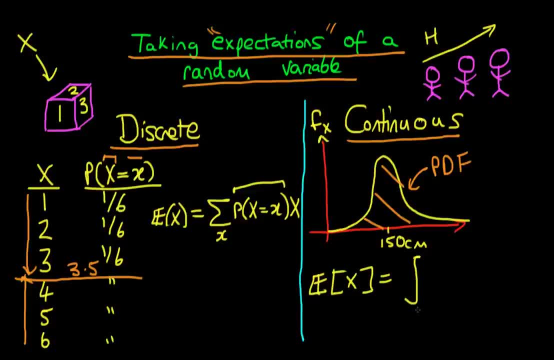 represented by this sort of p of x equals x by a continuous function, because now our random variable can take on all continuous values, So that particular weighting is provided by the PDF which I've indicated by f of x here, And then all we need to do is we just need to multiply that by 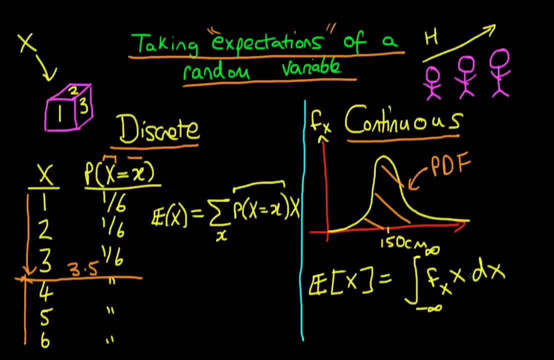 x and then integrate across x. So it's exactly the same sort of case as a discrete example, except now we don't have a sum, we have an integral, which is this sort of continuous version of a sum anyway. But what does it actually mean to integrate from minus infinity to plus?